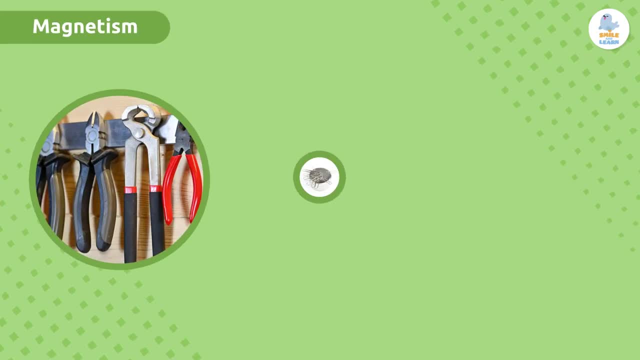 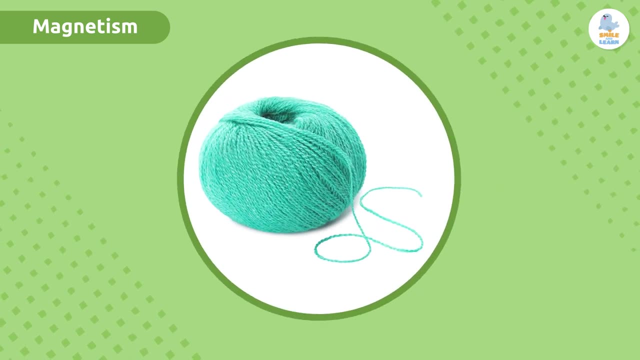 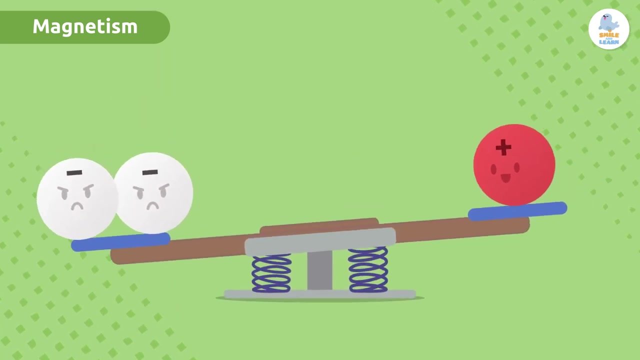 Now, magnetism is the property some objects have that attracts other metallic elements like iron. As you know, all matter has an electric charge. Normally this charge is electrically neutral, which means there is an equal number of negative and positive charges. 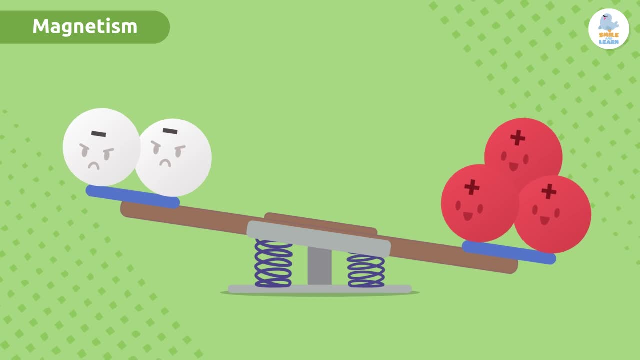 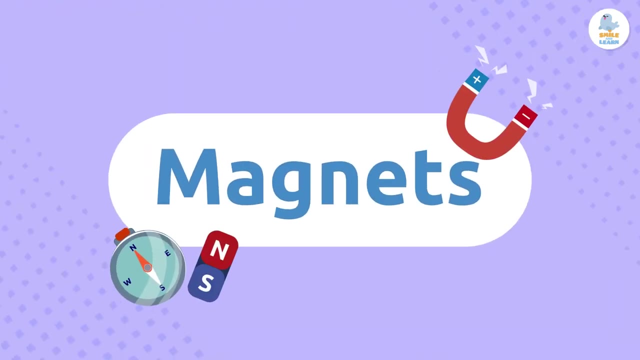 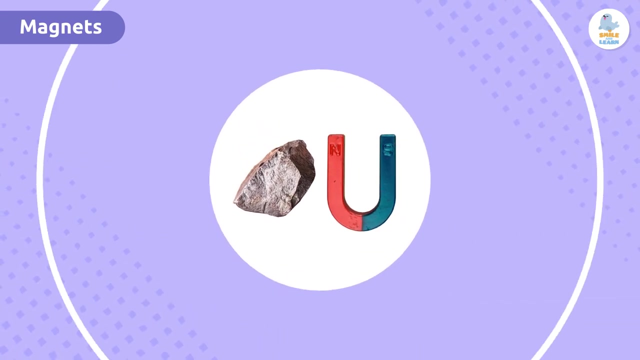 However, in some materials this is not true, and this imbalance of charges causes attraction or repulsion. Magnets can be both natural and artificial. One of their main properties is the ability to attract objects made of iron and other metallic materials. This is called magnetism. 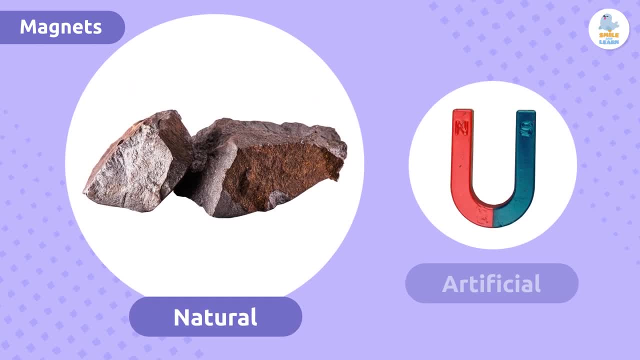 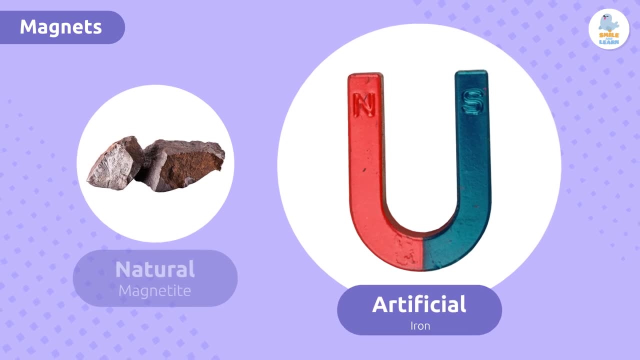 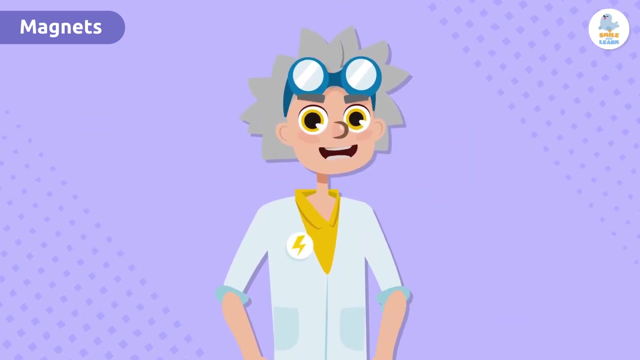 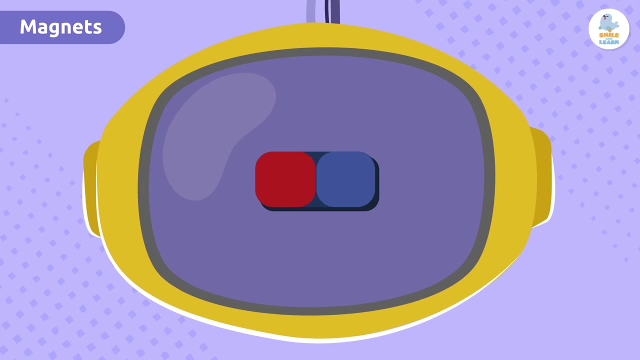 Natural magnets are found in nature. An example is magnetite. Artificial magnets are made by humans from different metals like iron or steel. So what are the characteristics of magnets? Come with me to discover them. Magnets have two poles, which we can find at their opposing ends. 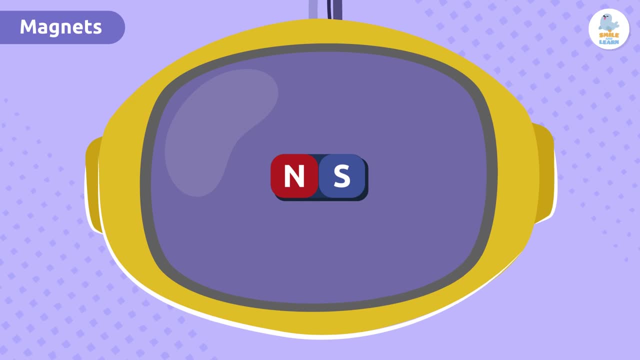 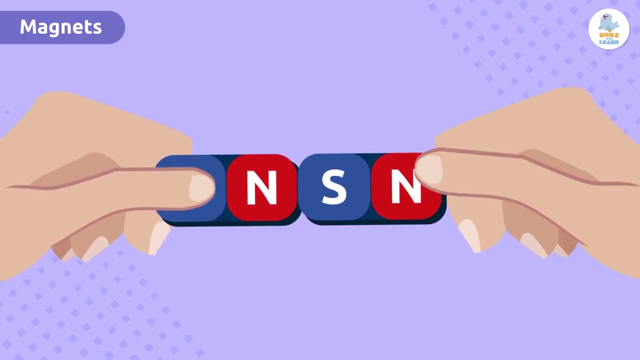 We call these ends the North Pole and the South Pole, and they generate a magnetic field. If we put two opposing poles together, they attract each other. This means that if we bring the North Pole of one magnet and the South Pole of another together, they attract each other. 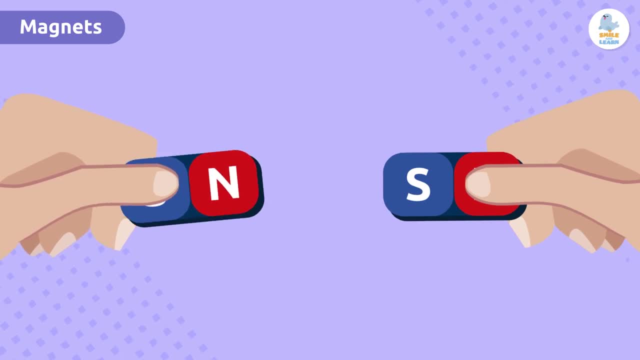 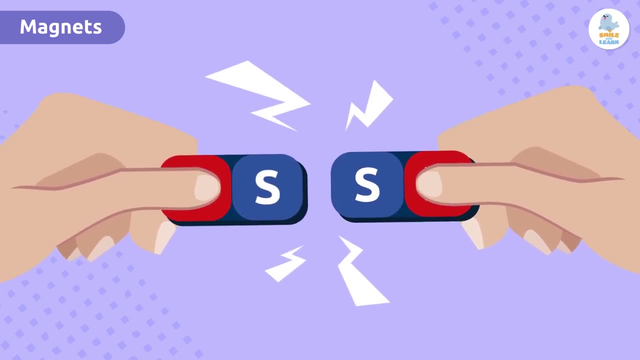 This means that if we bring the North Pole of one magnet and the South Pole of another together, they attract each other. On the other hand, if we put two of the same poles together, they repel each other. Pretty interesting right. 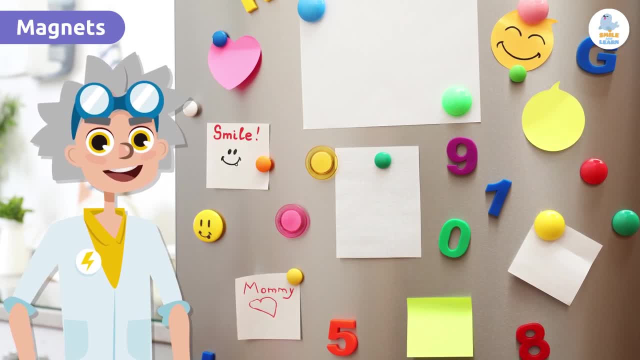 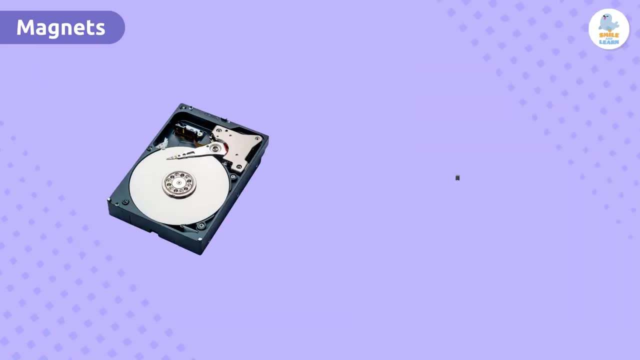 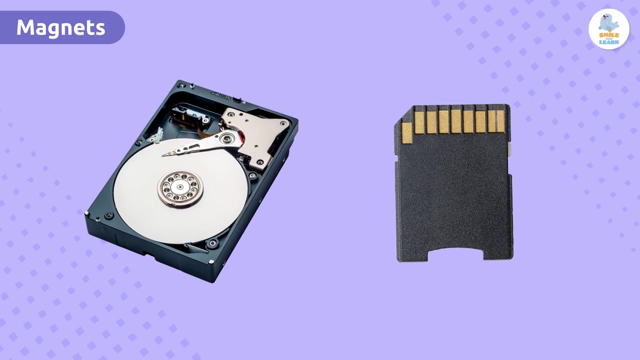 But magnets aren't just used to hang the shopping list on the fridge. They can be used for many other things. Let's take a look at some examples. Digital storage devices such as hard disks and memory cards use magnetic properties to store data. 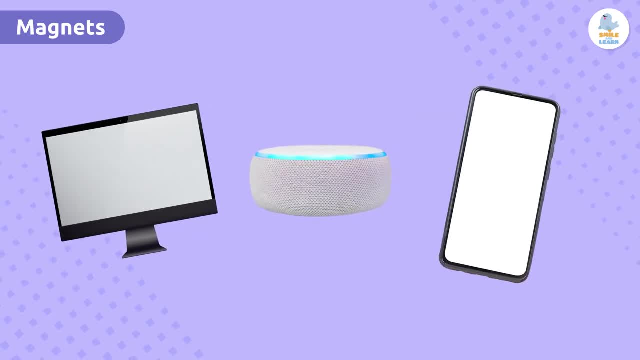 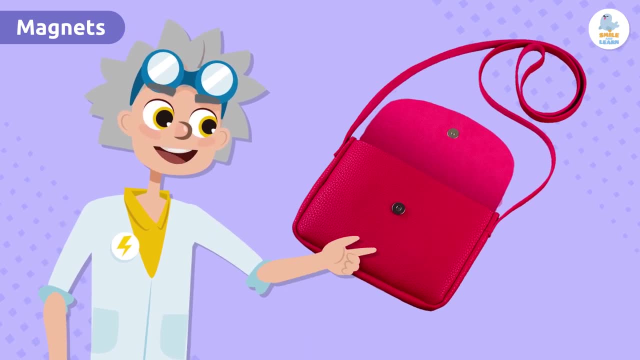 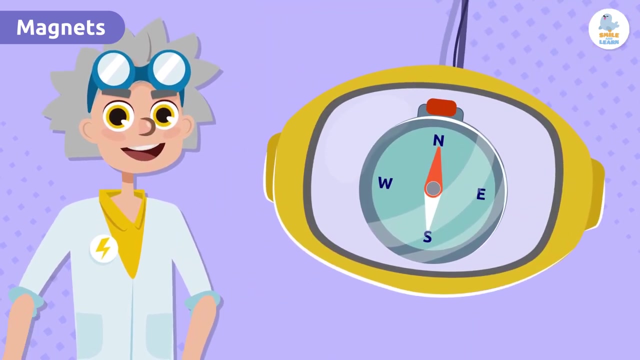 Screens, speakers and other electronic devices also have magnets inside them. They're everywhere. I'm sure you've probably seen magnets on the clasps of bags and purses before. right, Look closely. Did you know that compasses work thanks to magnets? 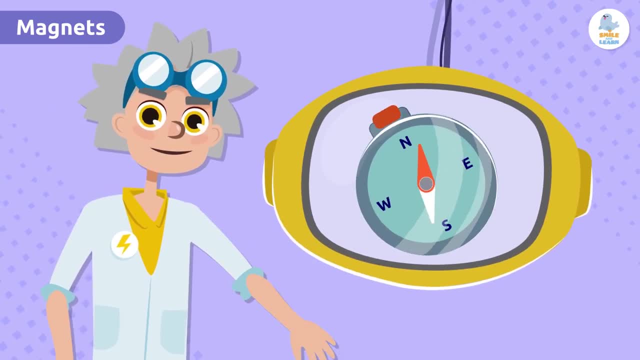 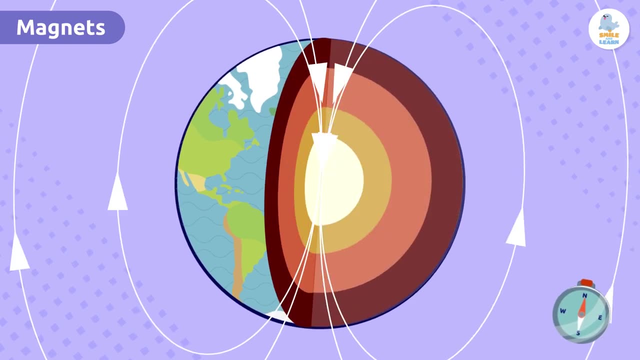 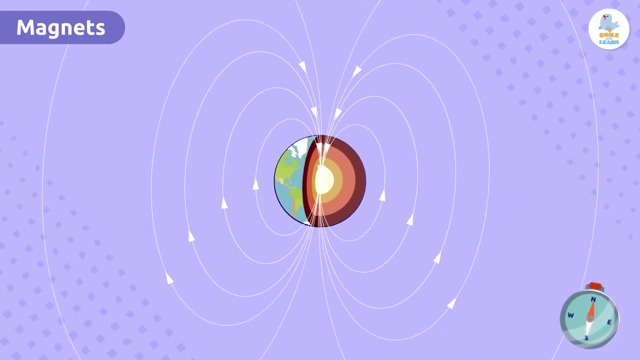 Magnetism is very important in knowing our orientation and location. This is possible because our planet has a magnetic field that starts in the Earth's core, Which is made up of metals such as iron and nickel, and extends through hundreds of miles of outer space.